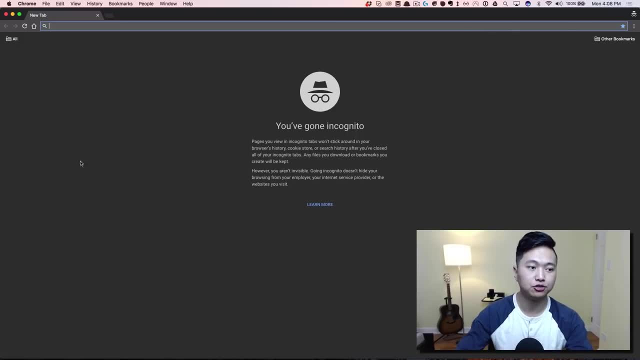 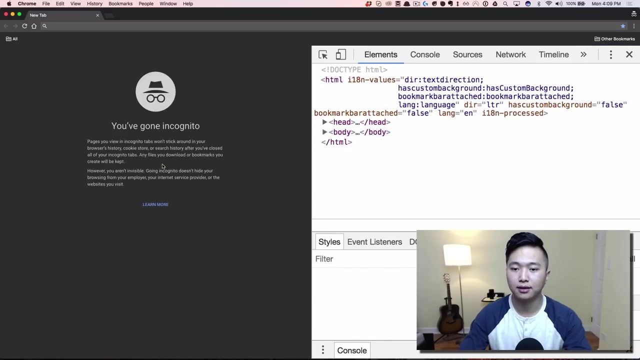 For example, you can just open up any Chrome browser and just right click and inspect. or, if you're on Mac, the shortcut shortcut is Command Option I. if you're in Windows is probably a Control Option I or Control Shift I, I forgot. but just do right click and inspect And you'll. 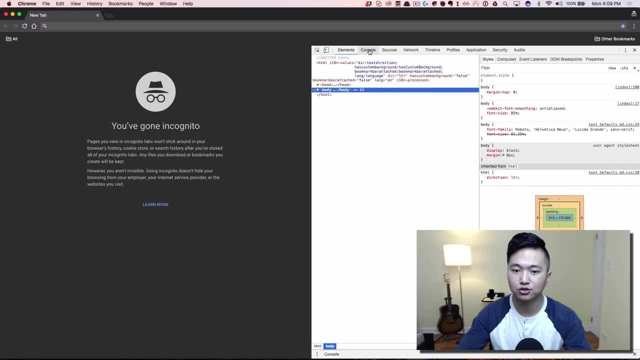 see this dev tools open and just click on this console tab And this is the JavaScript console, And a console is a program to run code. Okay, and this is the JavaScript console or the JavaScript code runner. okay, you can call that And here we can write. 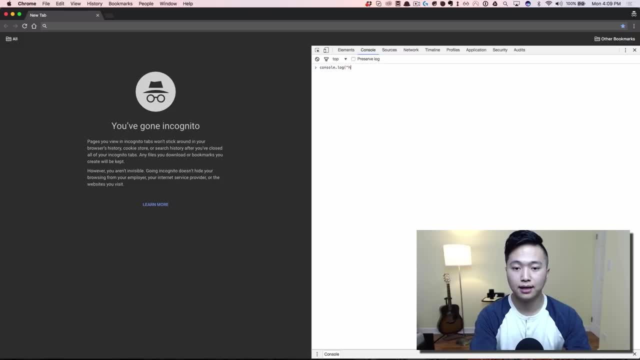 JavaScript code. So a console dot log. let's do hey man, what's up, And log that like we can do five plus five, right, And we can also do like built in functions, like hey man, There it is. 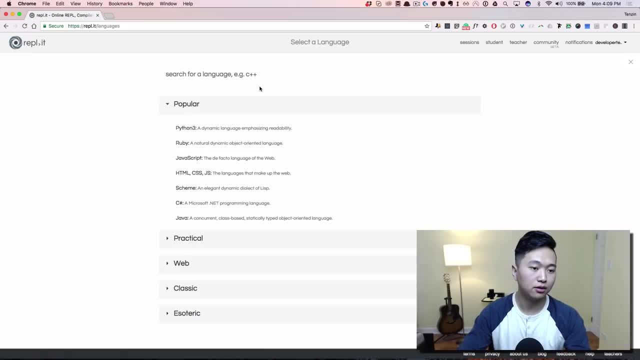 right. So this is where you can write JavaScript code. Another is another place where you can write JavaScript code is writeJavaScript in your terminal. So if you're on Mac, just open up, just search terminal from your spotlight or however you want, And just open that up. If you're on Windows, you should probably 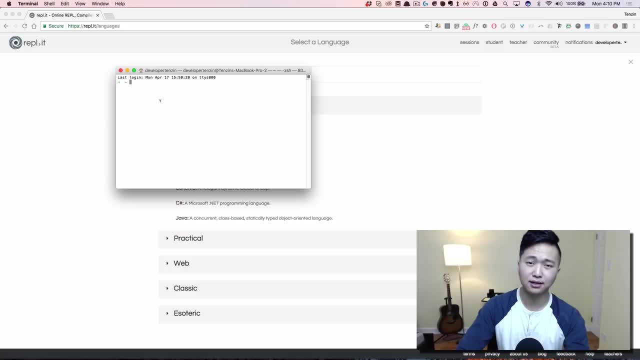 be using CMD or PowerShell, But I actually highly recommend you download a program called git, bash or sigwin or baboon. baboon is amazing. Okay, you guys should definitely get that If you have Windows and if you don't like the Windows command line stuff, we're not. 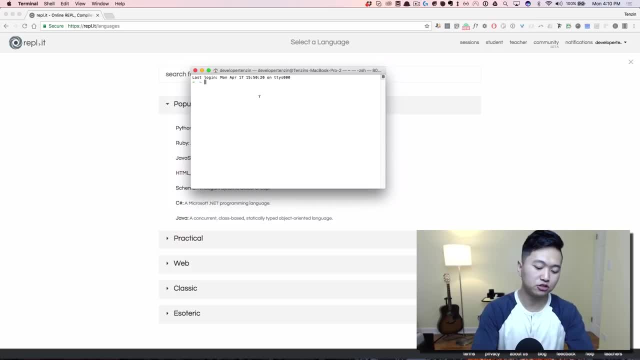 going to get into that in this video. So this is the terminal and you can just do node and that's it Alright. And if you don't have node, you can just install it just by googling how to install download, how to install JavaScript. Okay, So you can write JavaScript code here. 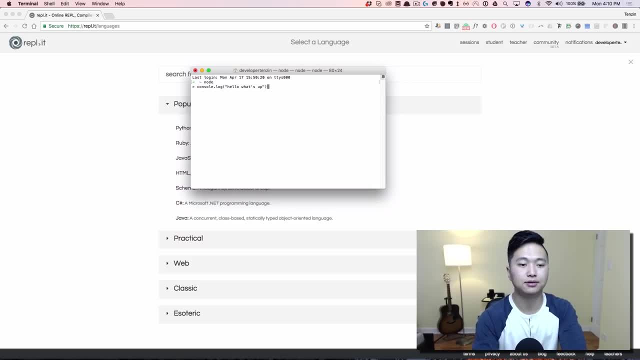 like consolelog. Hello, what's up? Right, You can do five plus five, five times five. So, yeah, this is another place where you can write JavaScript code, But we're going to be using a website called rebel it, okay, or EPL dot it, and it stands for read evaluate print loop, Okay, And this website 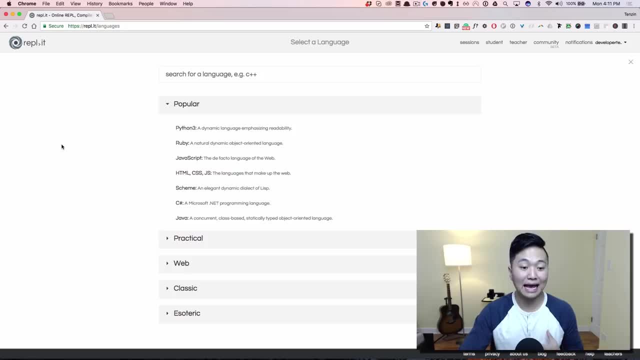 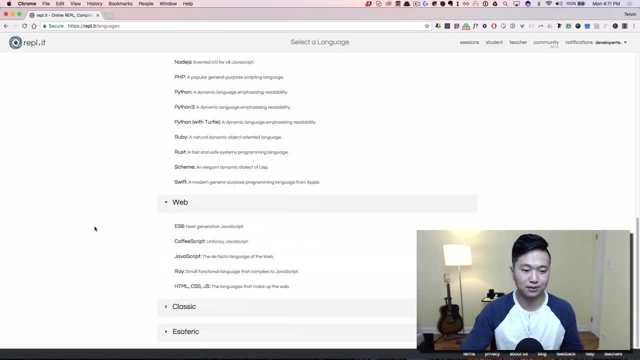 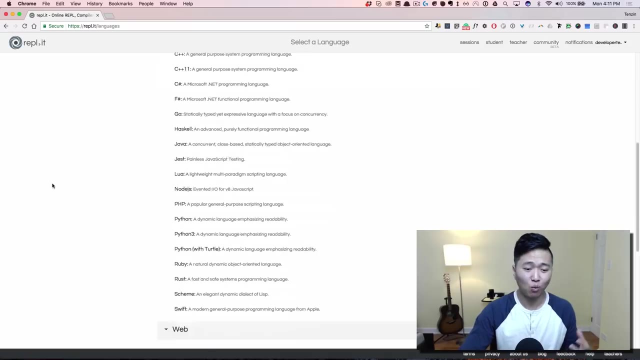 is just phenomenal: Like you can search up pretty much any mainstream language, like I don't know, like there's. like this website has all the languages that I will ever need to code and this website runs it okay, like Clojure, functional programming, web programming- like there's pretty. 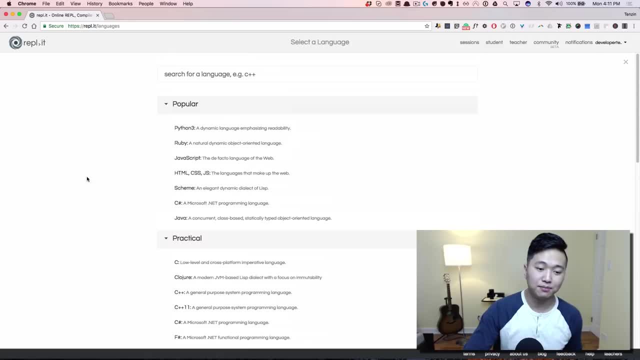 much anything like Java's even see, right. So it's amazing, But let's, let's, let's focus on JavaScript for now. So what you want to do is click on JavaScript, or just search up that JavaScript like this right, and click on JavaScript. Okay, so this window here on the 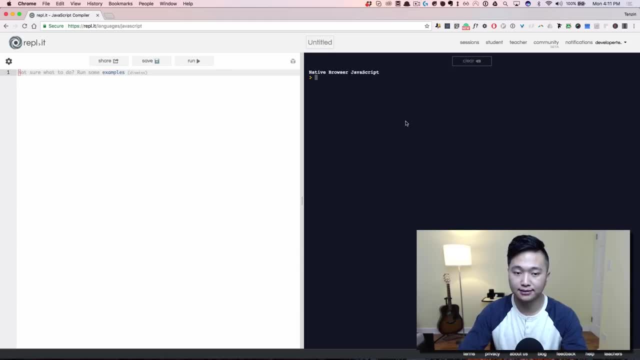 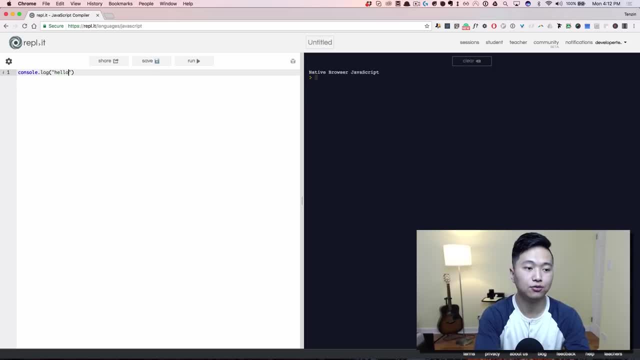 so we can do console dot log, Hello, And look at that right, It ran it and it printed out here. Okay, so the first thing that we're going to learn are data types. Okay, so what are data types? If we take an example of the real world, we have objects, right? 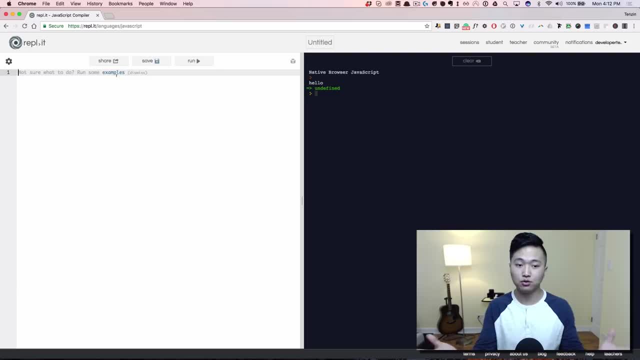 we have different types of objects, we have different types of computers, we have different types of tables, we have different types of mics. we have different types of webcams, right? So in the same way, in computers you have information. It's all virtual, like it's. 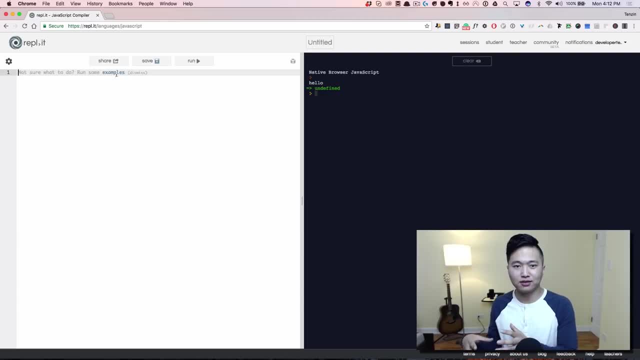 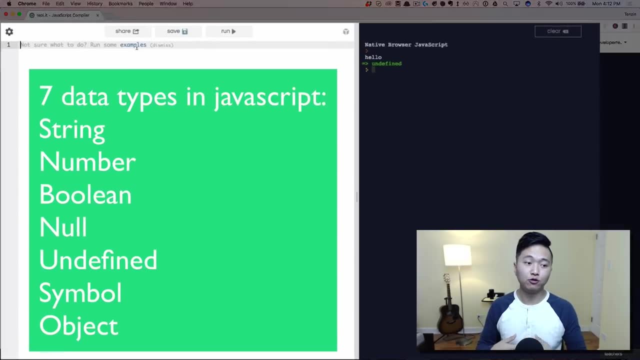 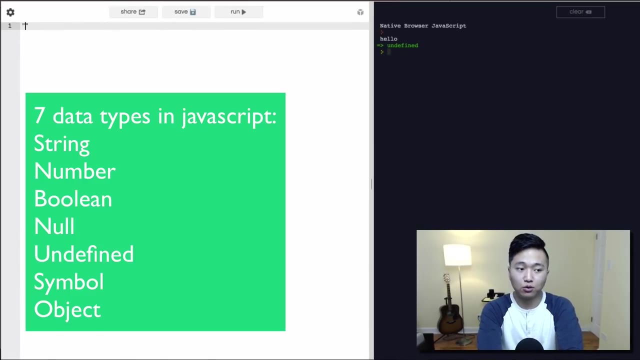 all digital. there's no like. then there's nothing that you can physically touch, So it's all data information. So we have different data types. So the first data type is called a string. Okay, so anything that's wrapped inside of double or single quotes is called a string. 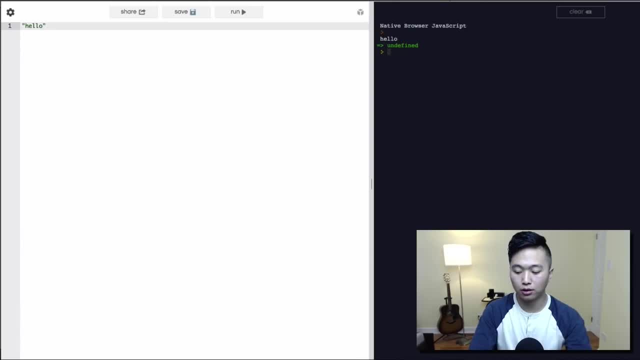 Okay, so let's do Hello, Or we can do a long string, any string that you want, like the walking dog is pretty messed up. Okay, that's another string. All right, And the function that the thing that I was using earlier, console dot log, right. 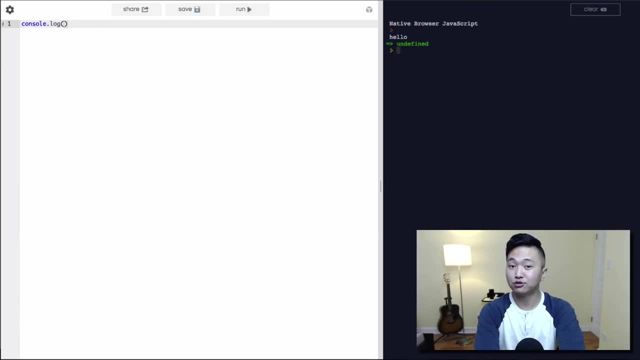 this thing is called a function. Okay, right now don't ask me what a function is. we're going to touch on that later- But for now, just know that it exists And the purpose of it is. whatever you write inside of these two- parent, parent parentheses. 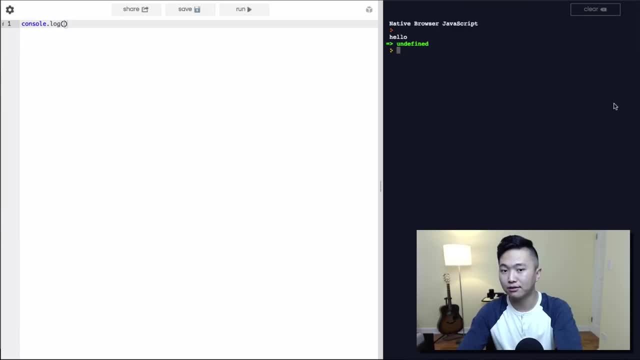 it's going to print it out to the screen, right here. it's going to log it out to the screen, Okay? So if we do, Charles is amazing. There it is. Charles is amazing, right. So it just prints it out. So we have a string called Charles is amazing And it's just printing. 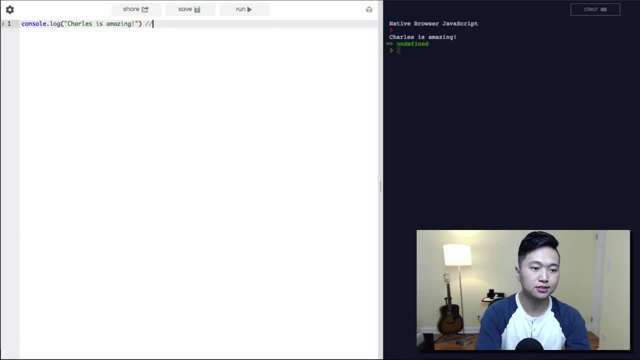 logging that out to our screen. Okay, so this is a string And the thing I just wrote. this is called a comment, And comments are things that you can put in your code. that has pretty much no effect on the code itself, But it's a note for yourself, right? So now we can tell that this is a string. 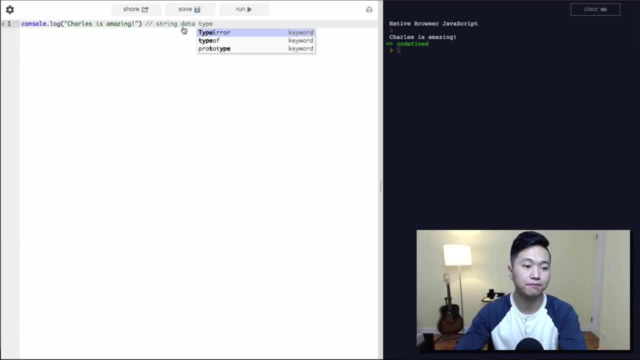 data type, right, So we can kind of like, this is a string data type, Right, So we can, you know, write string data type. okay, And let's just write it on a new line, probably above this guy. 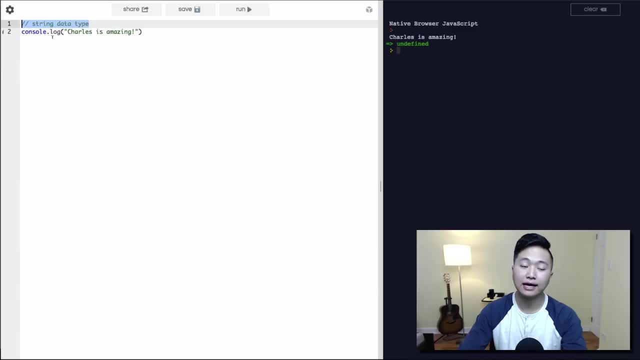 And that's what comments are it just to document what your code is about basically, Okay, that string data type and next data type is called a number And numbers. right, just like numbers. you know, you just type in numbers like 4834382.. That's a number and we're printing. 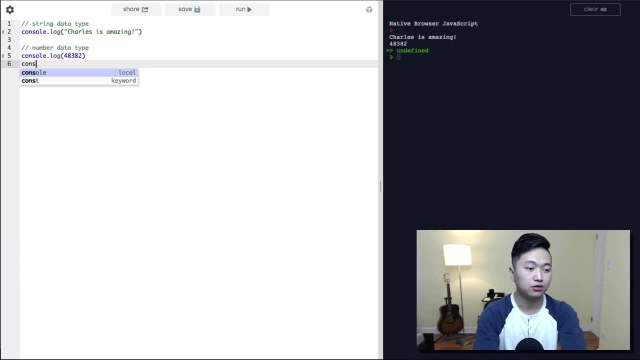 that out to the screen, logging that out to the screen. Now you can also have decimal numbers: 3.1416, a pie right And that's a decimal number in other languages. These two are different data types. like this: one is called an integer because it's a whole number, And then for decimal numbers, 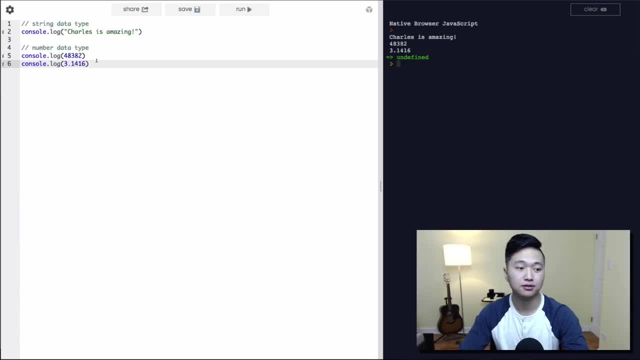 you have float data type, But in JavaScript you don't. you just have a number data type, just one right, real simple. And then you have something called Boolean- Okay, data type. So Booleans can be either true or false. That's it All right. And these are. 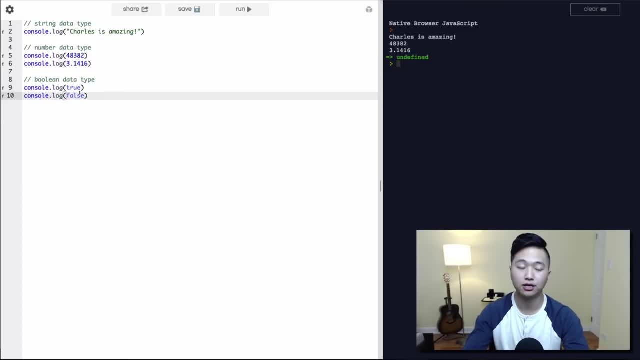 used to check if something is true or not later in our program- And we'll go over examples later how we would go about using those. So so, so far we've gone over string numbers and Booleans. But before we talk about another data type, I'm going to take a little tangent here and talk about 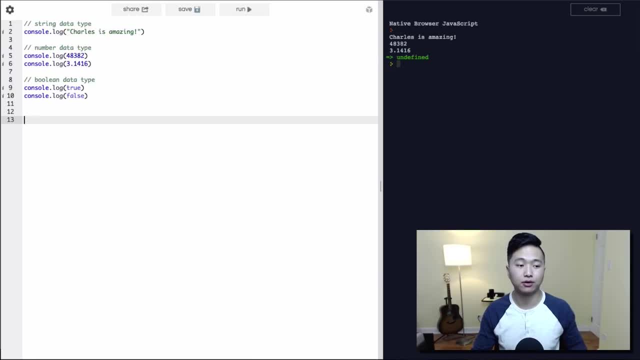 something called a variable in programming. Okay, what is a variable? So let's first write a variable. So var name equals john. So what? what the hell did I just do? So this is how you create a variable. We're with a var keyword And this is the variable name, and you're assigning that. 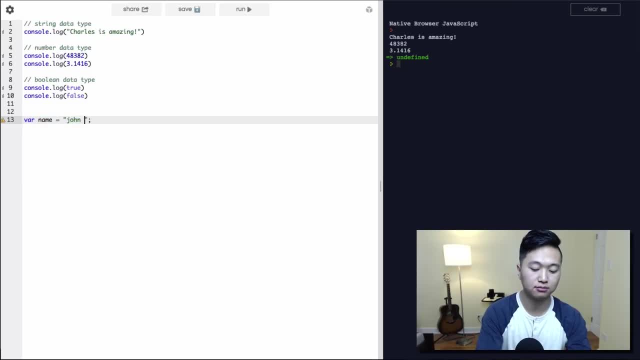 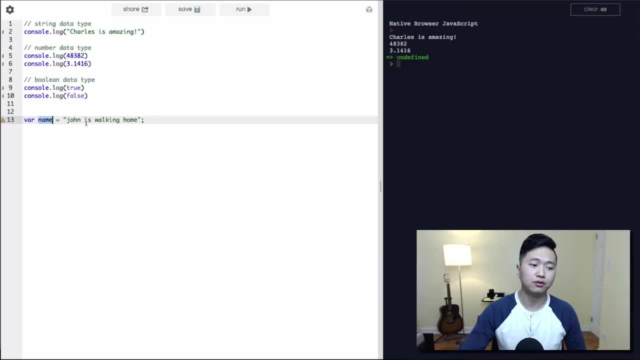 one, one, one, one, one one. So what is a variable? Well, variables are things in programming that store information, temporary information, And later on, if you need that information, you would just call it. you can get that, get access to that information, just by that. 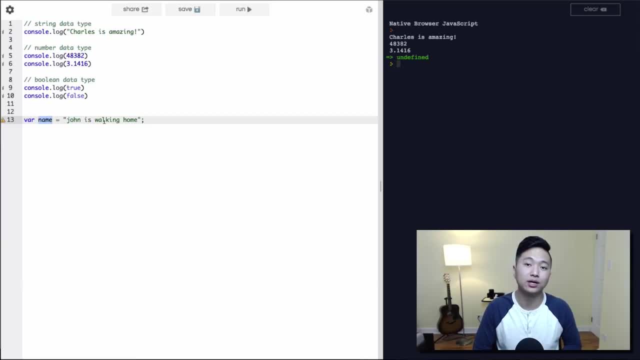 variables name, not, we don't have to remember what is inside that variables name, So you can think of it as an empty box, right memory box, and it just stores information, So So it doesn't have to be called name. it can be anything like mango, Japan, like anything. 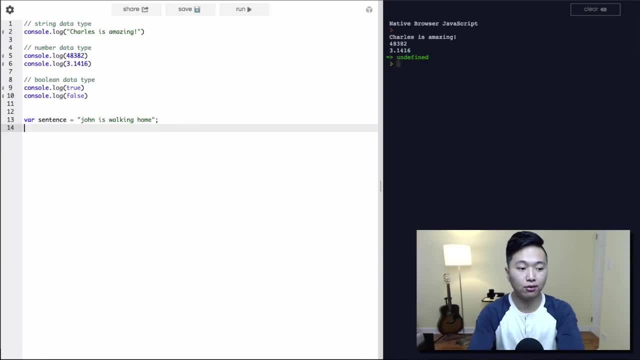 right, Let's call it a sentence in our case, And we can now log that out to the screen. There is john is walking home. right, We're console dot logging sentence And it goes. Oh, sentence is just: john is walking home. 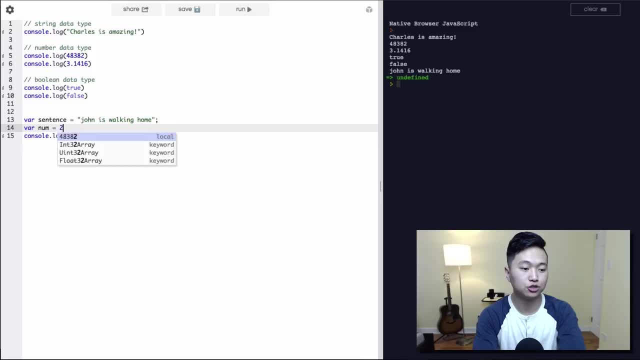 And now we can also store numbers and boolean. So like: num equals 23,. right, So now if we do like a new line console dot log, num will be 23,. right, There, it is Okay, And of course it can store. we can also store booleans and variables, but you get the idea. 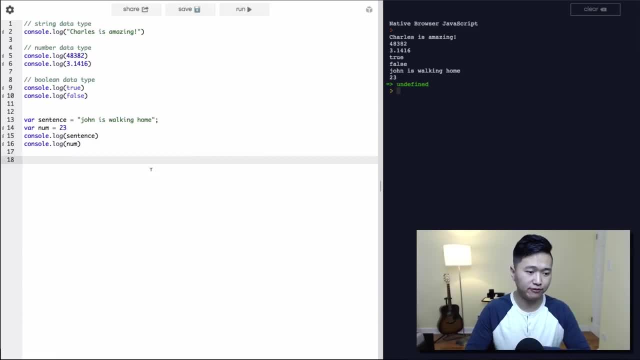 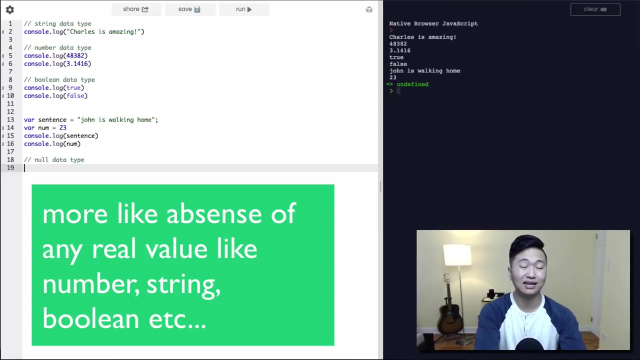 Okay, now that we know what variables are, let's keep moving And let's talk about another data type called no. Okay, so what is no no data type? And no Basically means something doesn't exist. okay, it's non existent. 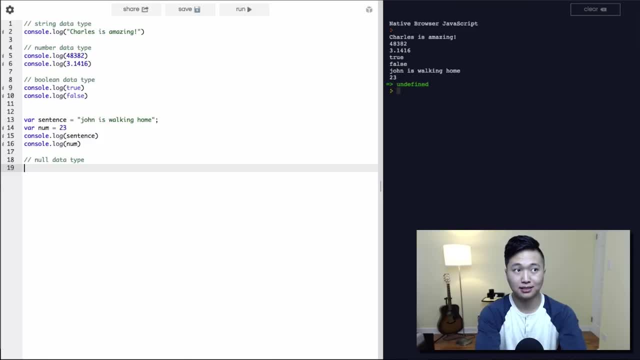 So you can actually make a variable and assign it a value of no. okay, so we can say, if our empty stuff equals null, And we can log that out by doing empty stuff and it will log no, right, So no basically means something doesn't exist. okay, it has a value of nothing, okay, doesn't? 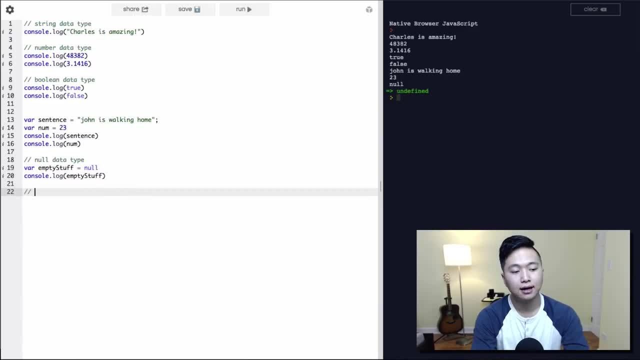 exist, So let's keep going. Another is undefined. Okay, And this you will see pretty often And it's very important that you understand what it is. Let's go over it. So let's: undefined data type. undefined data type basically means that a variable is not. 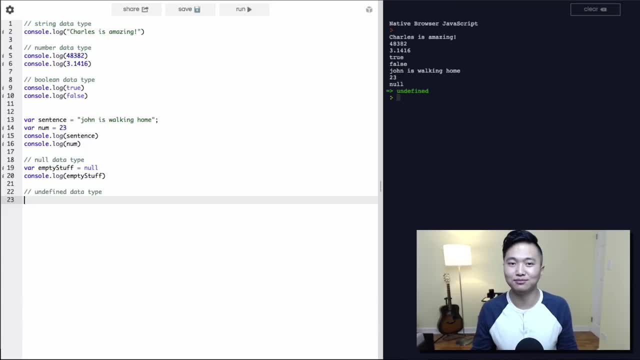 defined right. So you're like: what the heck do you, what the hell do you mean? Tenzin? It's of course right, undefined, But so undefined. Let's say we create a variable. Let's say we create a variable. 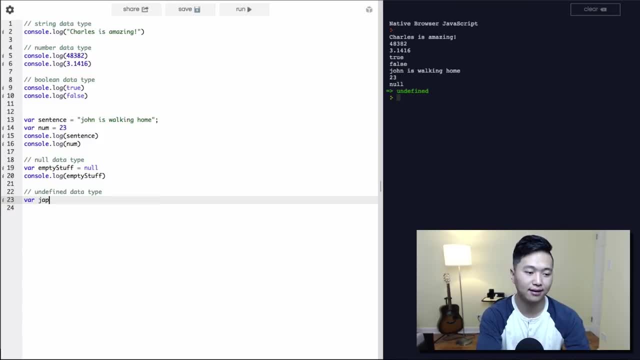 Let's say we create a variable here And I'm going to call this Japan, okay, And of course we can assign it something, some value, And let's just say: Japan is very beautiful, okay, And if we log that out, of course it will say: Japan is very beautiful. 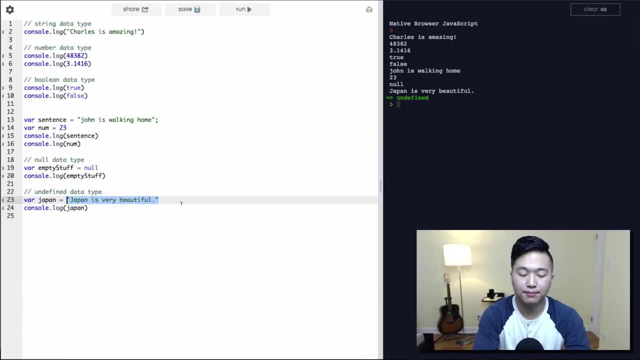 But we can also not make it equal to anything and just stop right there. Now what we're doing is we're declaring a variable, we're not defining it. okay, So now this Japan variable has a value of undefined, And all data types, if they're not assigned by default, have a value of undefined in JavaScript. 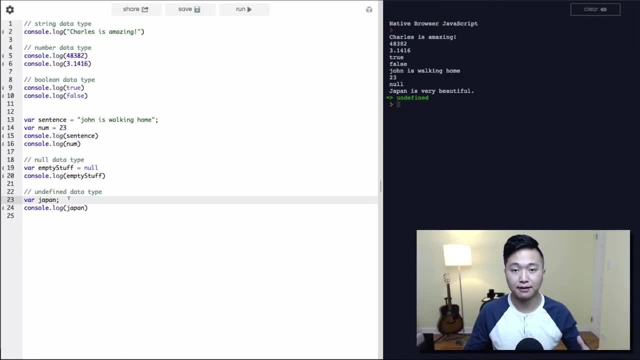 okay, So they all have a value of undefined from the beginning by default. And if we assign it something now, that value changes. So sentence here has a value of undefined Initially. but we said Oh var, sentence equals John is walking home. 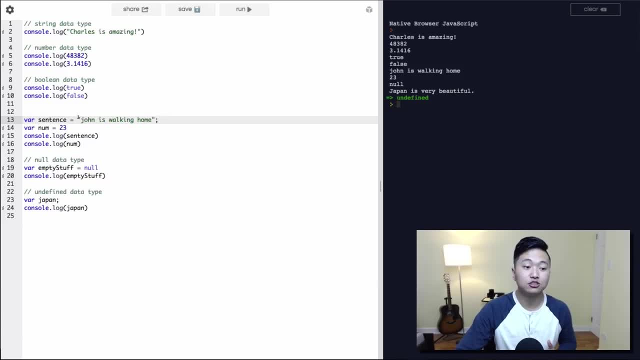 So then, the value of a change to from undefined to John is walking home, And that's why, whenever you do console dot log sentence, it did, John is walking home, All right. And there's a reason why you see this green undefined here. 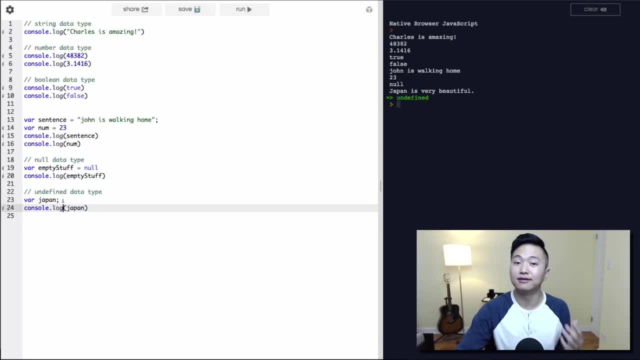 We're not going to go into that right now, But it has something to do with this undefined type. Okay, that's an undefined data type, Alright, So let's keep going Now. another data type is called symbol, But we're not going to talk about this data type, okay. 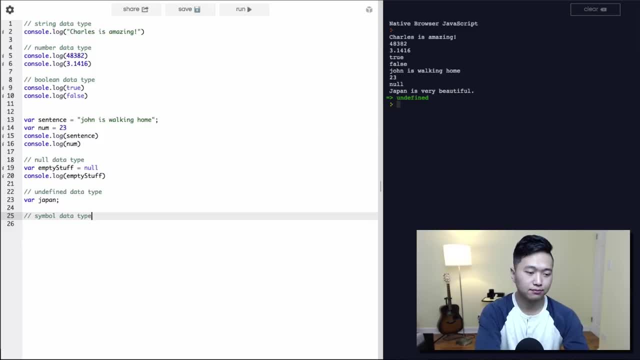 It's just not that practical for this video, because most people will never be using this anytime soon. If you're learning JavaScript, okay, Later on, when you do meta programming or more advanced stuff, then you might be using symbols a lot more, but for now, no okay. 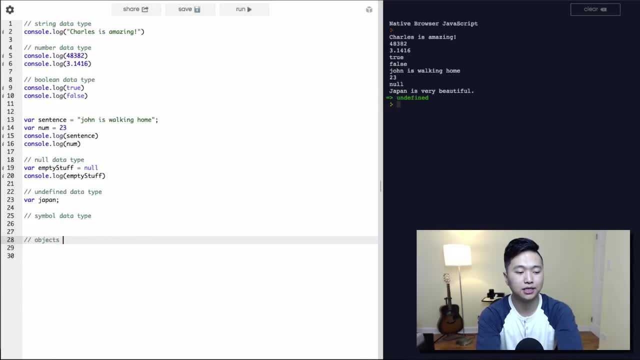 And now we have objects. All right, So objects are, they are, more advanced data types. okay, And we're not going to go too much into why they're advanced data types, But let's just see how they are created, Okay. 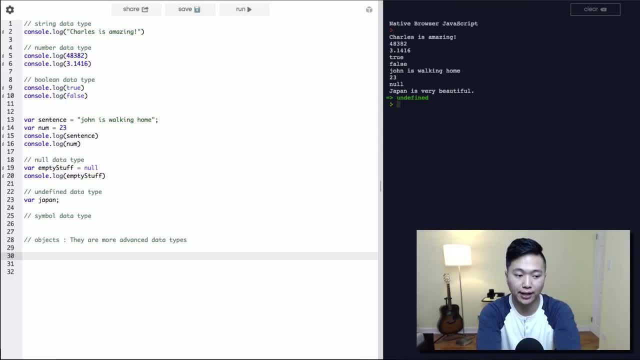 So there are many types of objects. The first one we're going to go over is called an array. So array. So let's go over arrays. Arrays are a way to store multiple things. So let's say we have a variable, A variable called fruits. 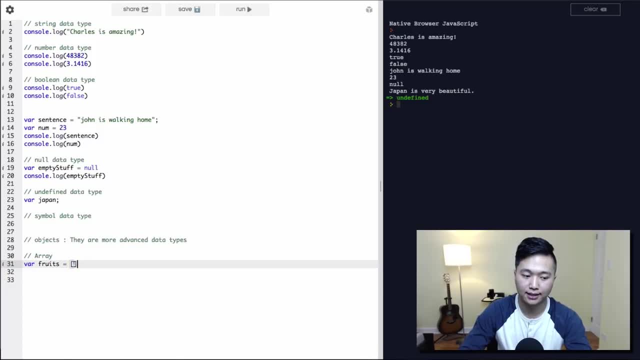 And arrays. we create that with opening and closing brackets, okay, So we can have apple and then comma, cherry and banana. So now we have a fruits array that stores three things, right, three strings, and apple, cherry and banana. 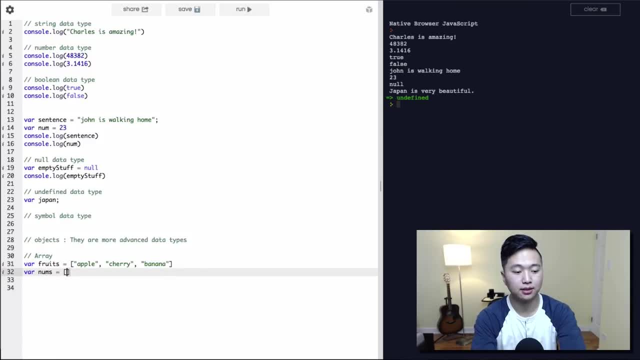 Another. let's create another one called nums, And we can have 123.. Right, Let's console dot log those like fruits, right? And we can also include other data types inside of our array, So we can do true, a Boolean, false numbers as well. 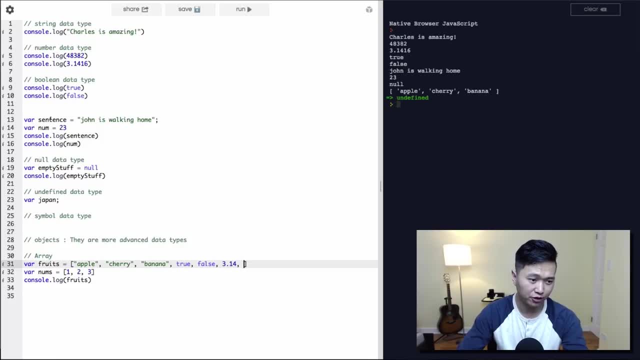 And even variables. So we have a variables variable called sentence here equals john is walking home. Now we can put sentence in here, Okay, And now, if I log that out, there is right now we have apple, cherry, banana, True, false 3.4,. john is walking home. right, because this gets evaluated. 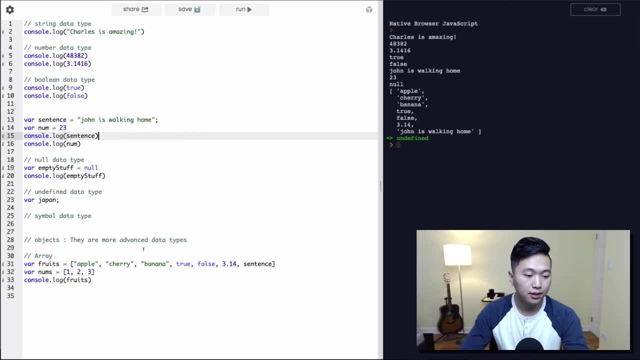 And we know that sentence is: john is walking home. So that's an array And another is object. So now you're wondering: hey, Tenzin, we. you just said we're going to go over two different types of objects and we went over array. 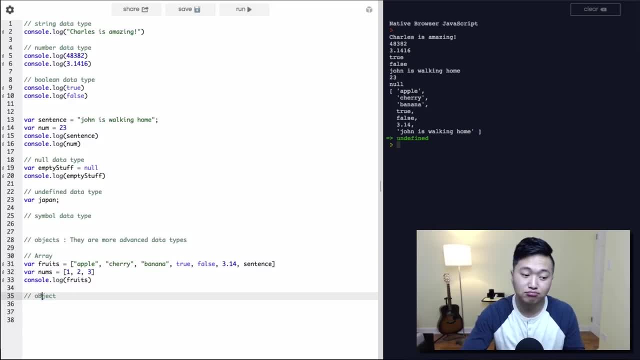 So now the second type is an object as well. You're correct, This object, okay. So really what's happening here is array is just an object, Okay, And right now there's no point of talking about this too much, because it really takes. 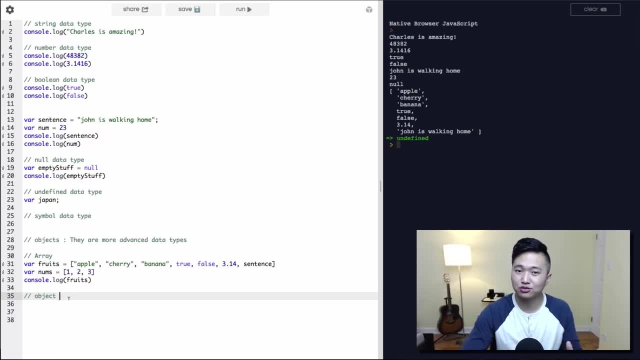 some time of programming before you can actually understand what an object is and how, how. everything is an object, And you might hear this from so many people, but most people understand it after a long time of programming. then they realize: oh my God, everything is an object. 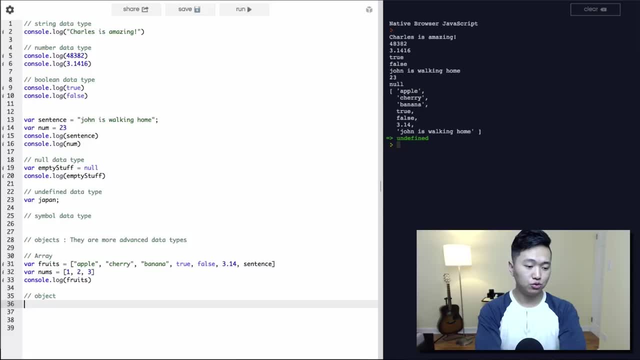 But that's not. that's another story. But to create objects. Okay, So let's say, you use the curly braces. okay, so you let's say we have john and we can use curly braces, And now we can describe what that object is about. 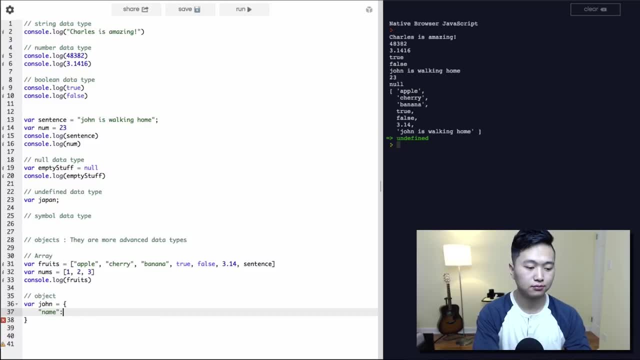 So we can do name Johnny bones Jones, right, And then we can have age and the value to a number, let's say 88. And then we have profession: Okay, UFC fighter. okay, maybe not 88.. 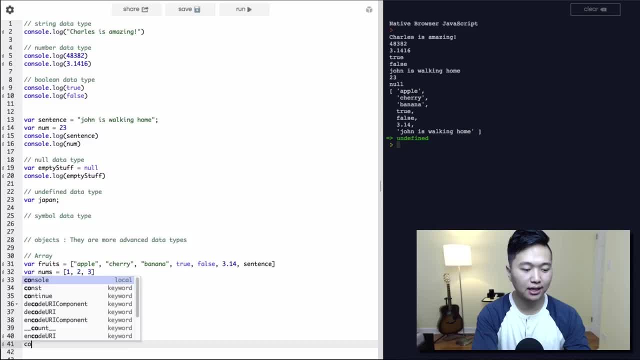 Let's say 31.. All right, And now we can console dot log that as well. Okay, john, there it is an object is another way to store multiple things. Okay, so we have john variable that stores an object, right. 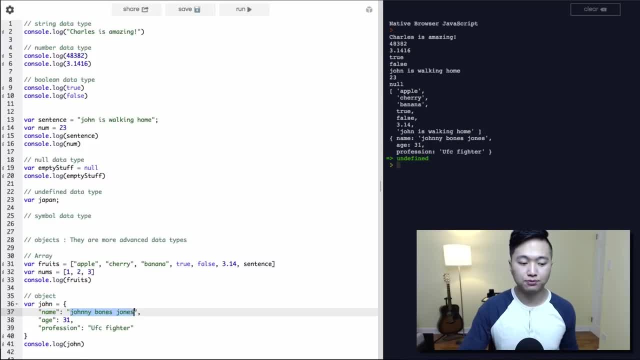 And we have a property called name, with a value called john bone Jones, property called age with a value of 31.. Nice Number type. And then we have a property called profession And we have a value of UFC fighter And we can also have, like say, hobbies, right. 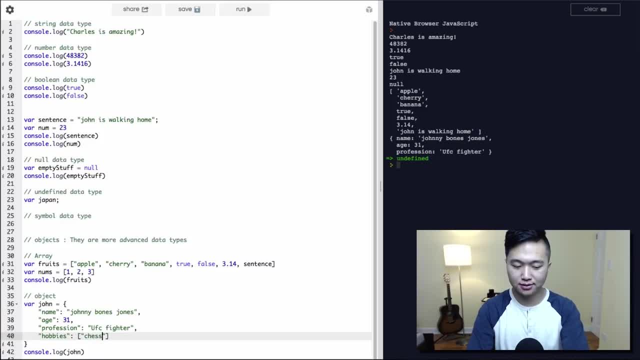 And we can do chess, snooker, fighting, right. So a value can be an array as well, So an array inside of this object, right. So objects are very flexible data type. They're really structured data structures, but we're not. that's another story.